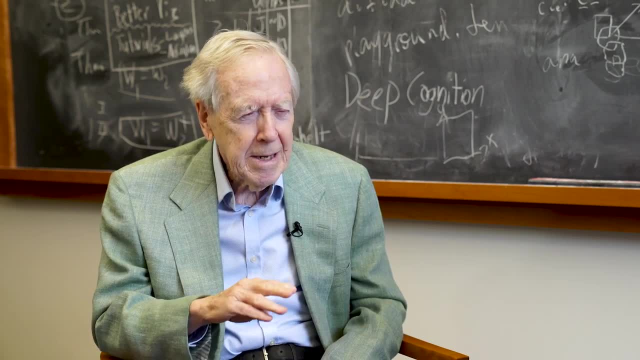 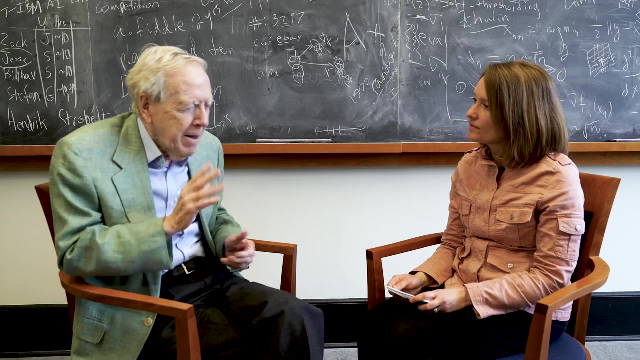 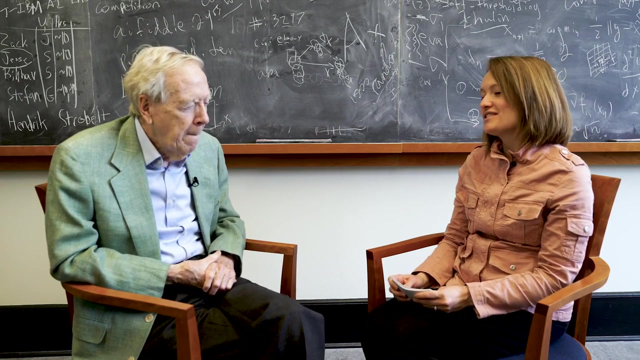 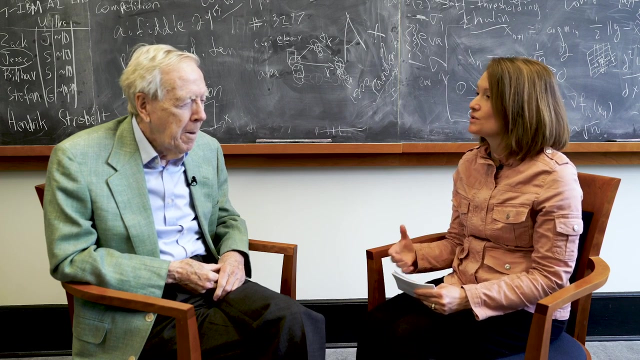 Because this class has to be sort of thinking with you And that's yeah, that's my thought. I don't know if I achieve it, but I think it's the goal. Mm, One of our- Yeah, One of our- users on OCW noted that during lectures you sometimes ask rhetorical questions or maybe feign confusion as a way to work. 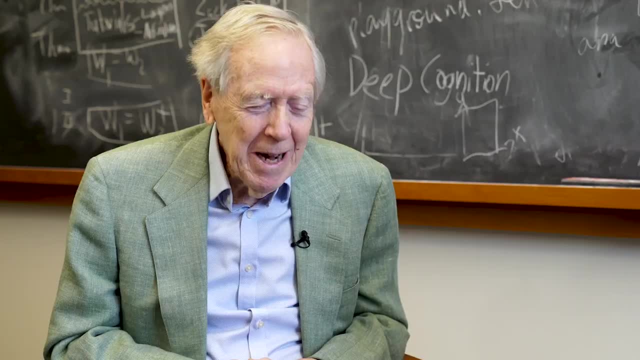 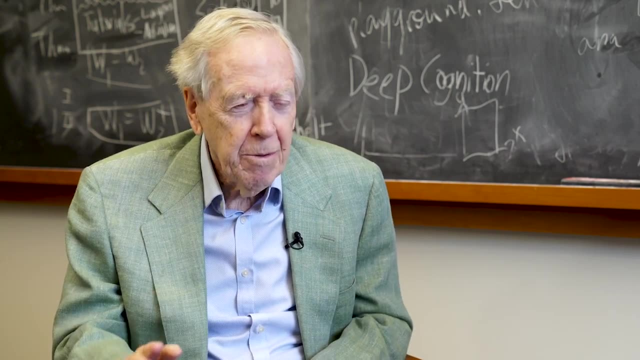 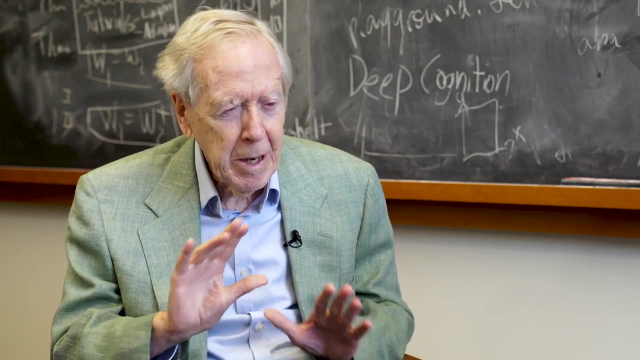 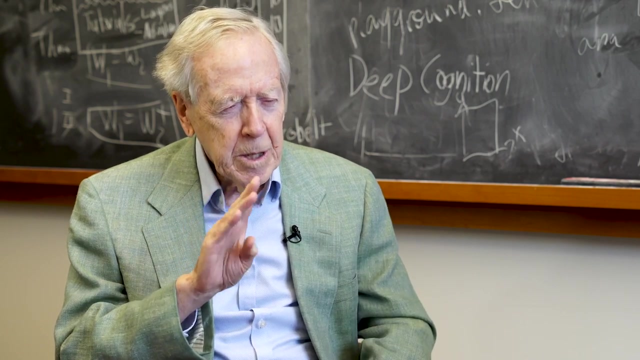 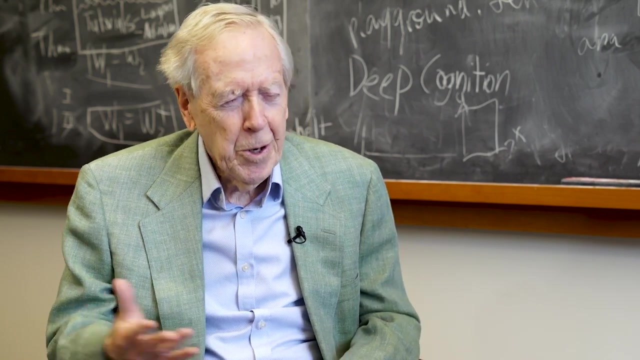 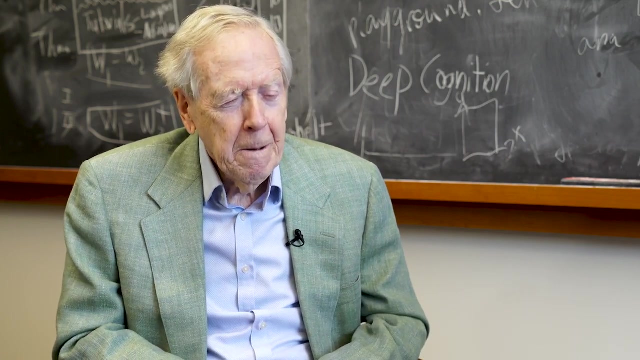 Feign confusion. I'm confused. Are you Well? no, Okay, Well, no, it's probably true. That's maybe part of not rushing through it but getting this. so I'll pause to at the critical point maybe, and give you have to give time to see, okay, what's the next step. You know it's mathematics is beautifully ordered and sensible and logical, and linear algebra is not too difficult, But still you can't rush. You have to sort of see the idea a few times. 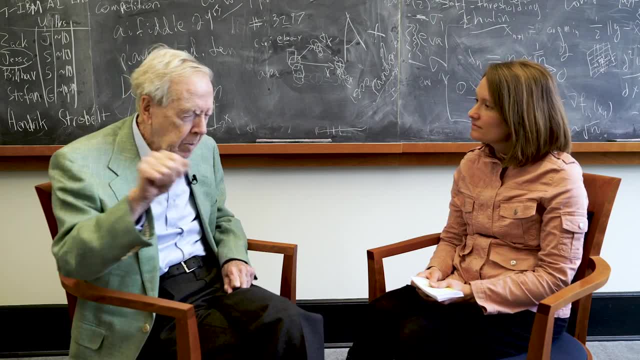 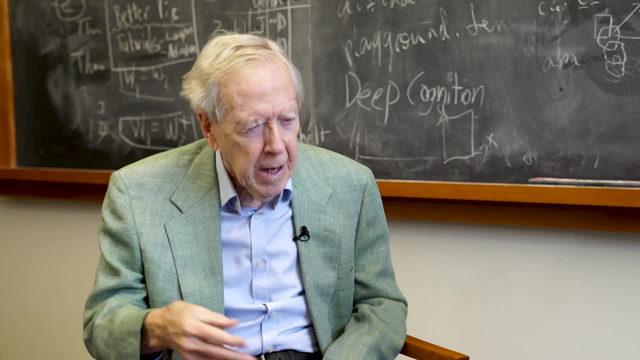 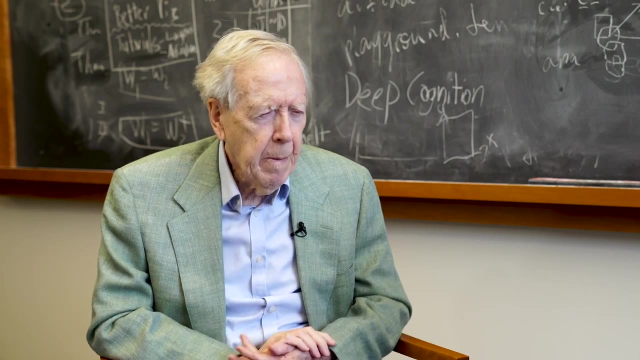 Mm-hmm, First maybe on the board as symbols, But not everybody picks up on symbols. Then you say what does it mean? And then finally, you say why is it true? But you don't say why is it true. Give the proof, The very first step. Yeah, you want to make people think: yeah, it is true. 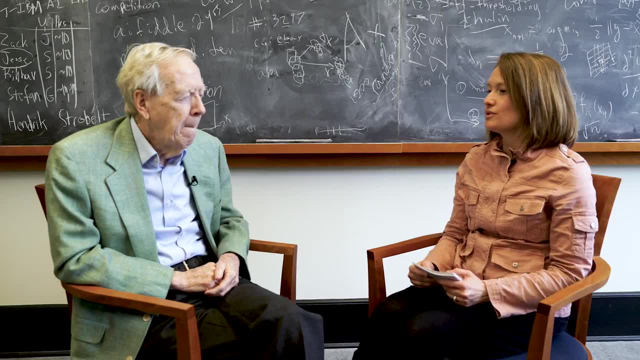 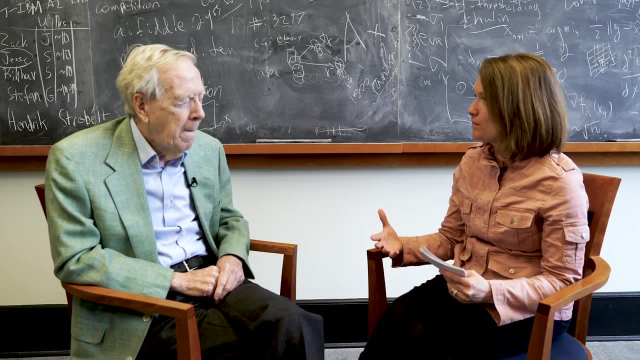 Mm Right, Others have noted that you do this thing where you display your Mm-hmm, Mm-hmm, your own thinking, kind of on the spot, as you work through problems. Yeah, Is there ever a risk in that for you? 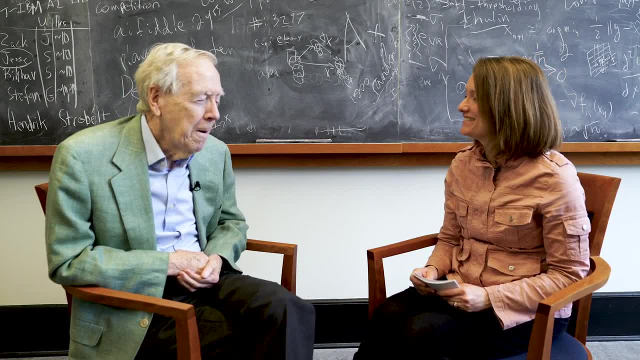 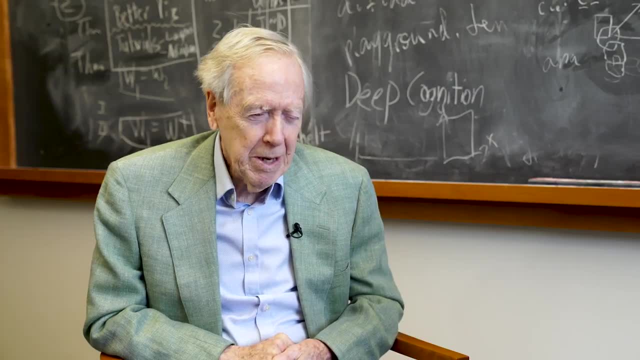 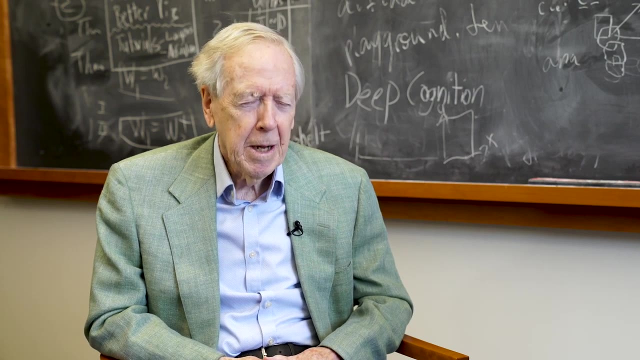 Oh, yes, And it happens that I lose the thread or I come up to a dead end where I don't know what I'm supposed to do next. But generally, especially in 1806, the basic linear algebra course that many people have watched, 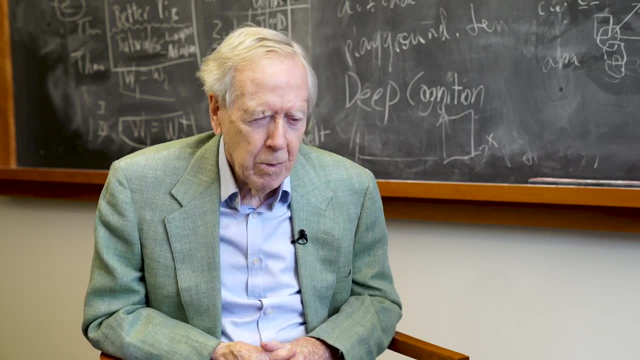 there I kind of get it okay. Sure, Yeah, I've taught it enough times to have a good chance of getting it right. Is this a strategy that you developed over time? You know lots of people are nervous to do that to. you know, make themselves vulnerable in front of a large lecture class like that. 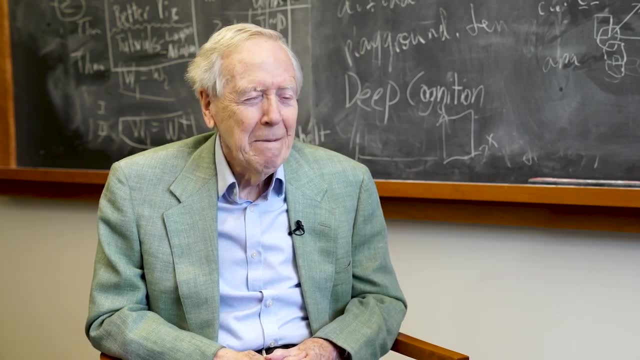 Yeah, But you're working problems in real time and demonstrating what happens when you hit a dead end. Yeah, Well, that's okay, because students are going to hit dead ends. so it's Yeah, Yeah, Yeah, Yeah Yeah. 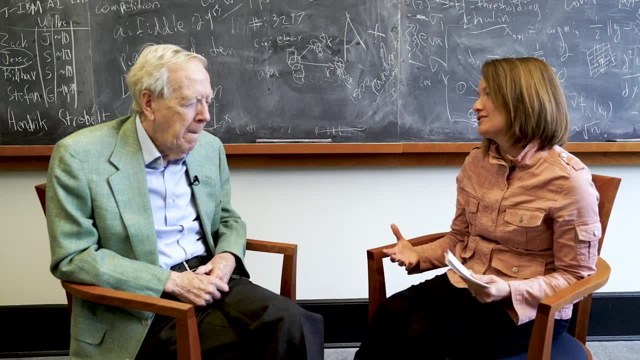 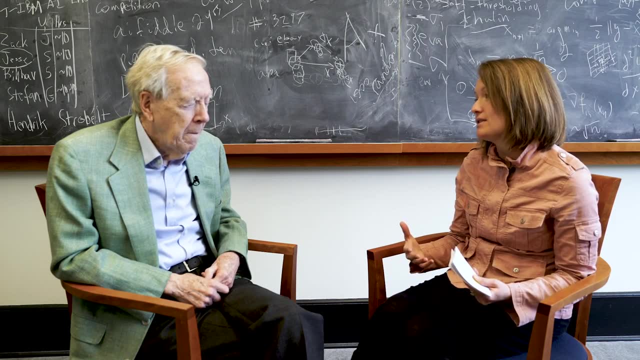 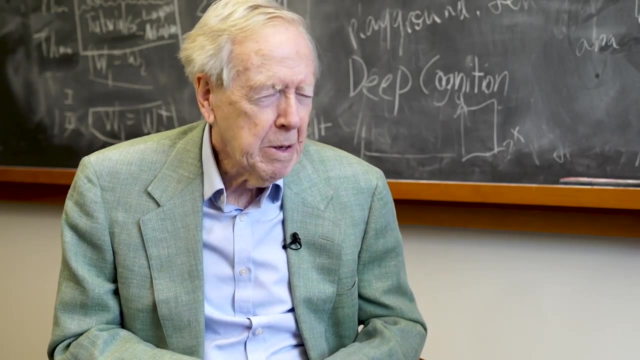 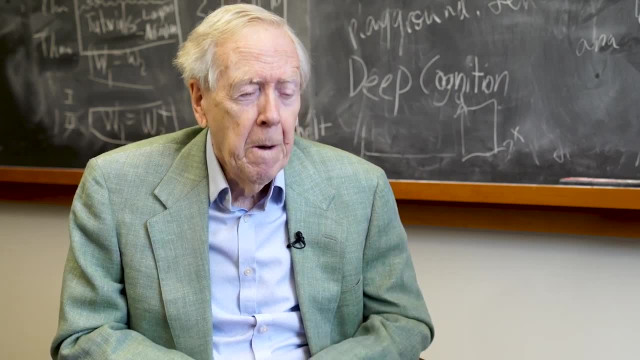 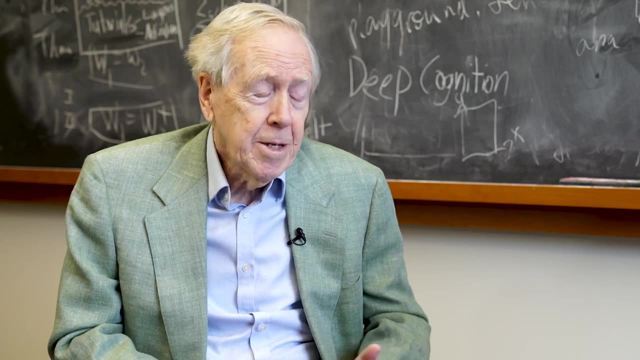 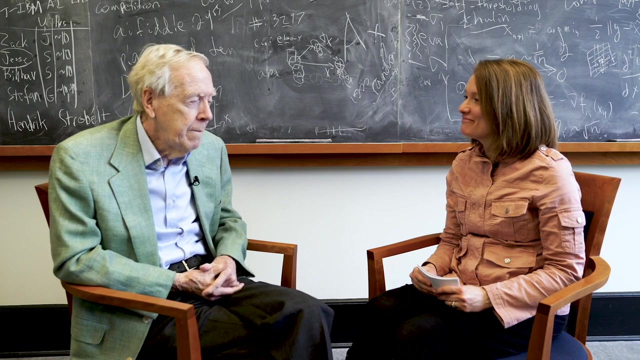 okay, maybe this is the way to get out of that, Right, Right, Ooh, Yeah. So essentially, I think the thing is: I like students, I like math, Mmm-hmm, And putting them together is just the best job in the world. 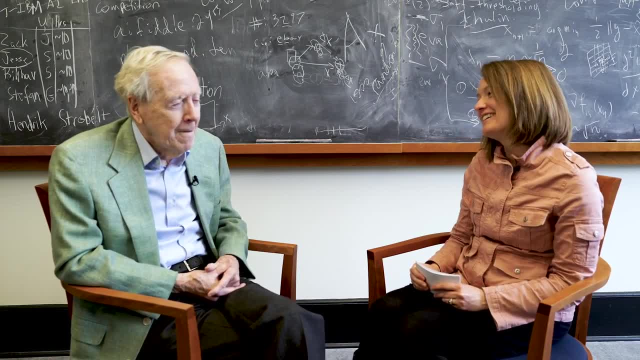 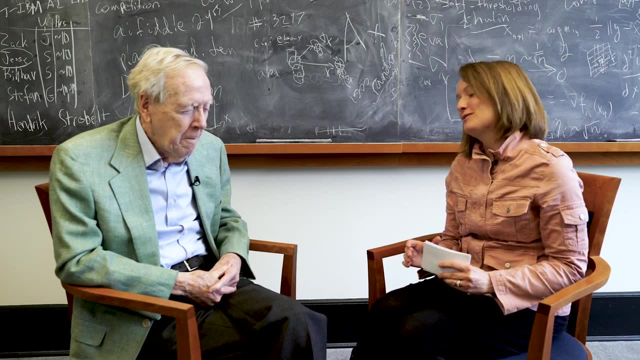 Let's talk about humor for a second. OK, I don't take it really like keep things in their Goss-given order and other like really funny things that people just love. So what's the role of humor in your teaching? 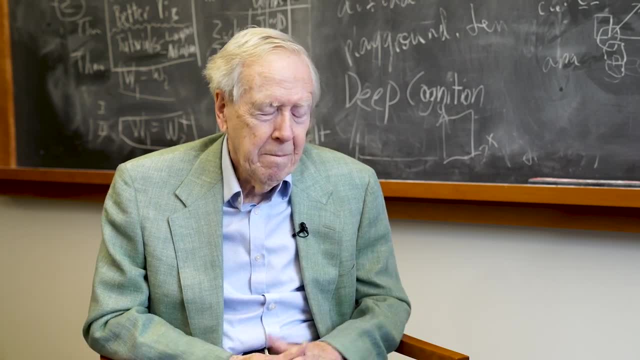 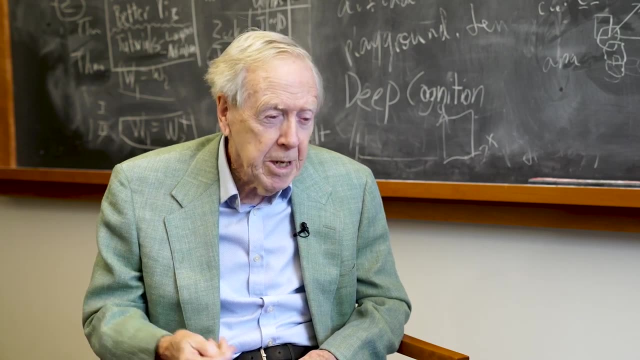 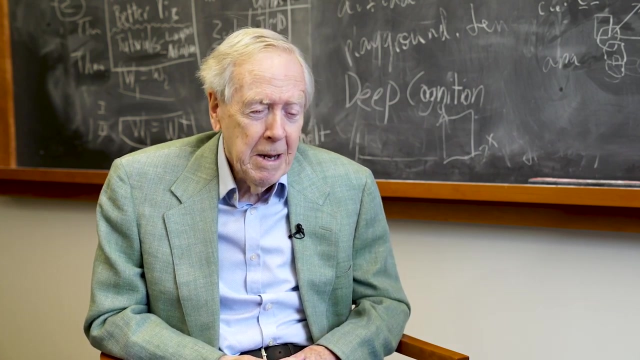 Well, it, maybe it's, which is what I'm saying here. it's. maybe the key point is to make it human. You know, you're a person like the student is a person. the book isn't quite a person, but it was written by a person, and to 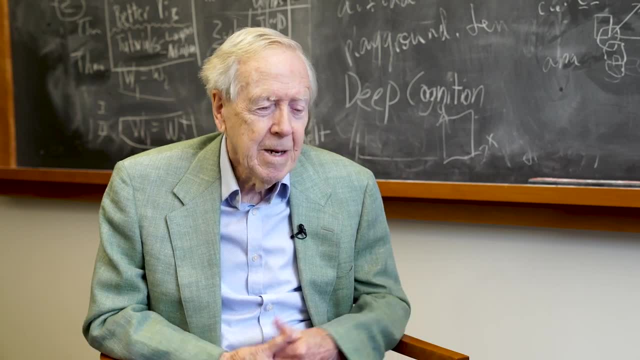 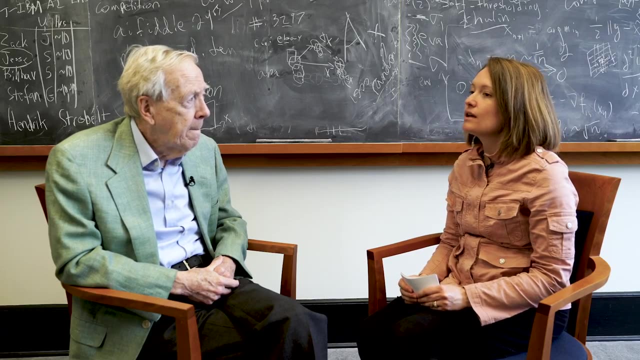 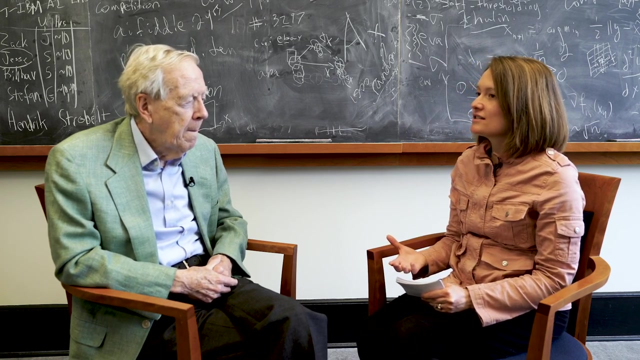 to see that it's just like a natural thing to do. yeah, yeah, yeah. So one of our users was thinking about how you teach complex material, how you convey it in ways that are comfortable for students, and the user was wondering: how do you know when to go into detail and when not to? 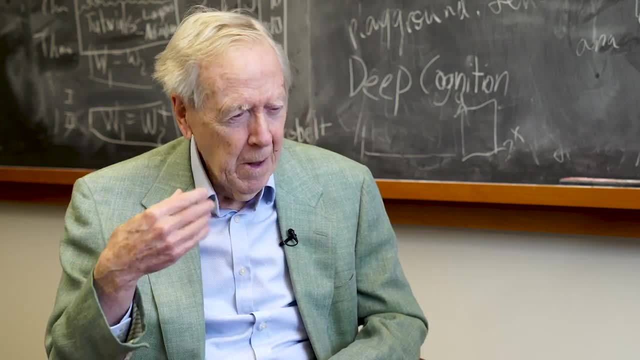 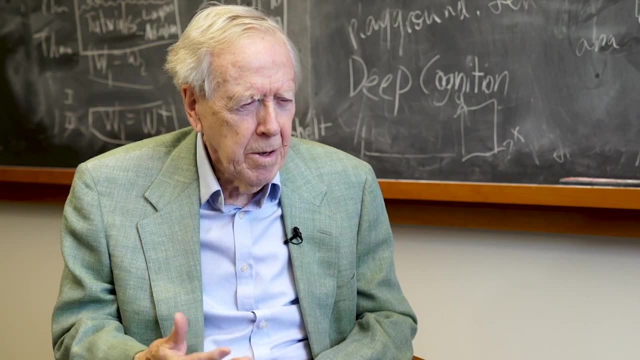 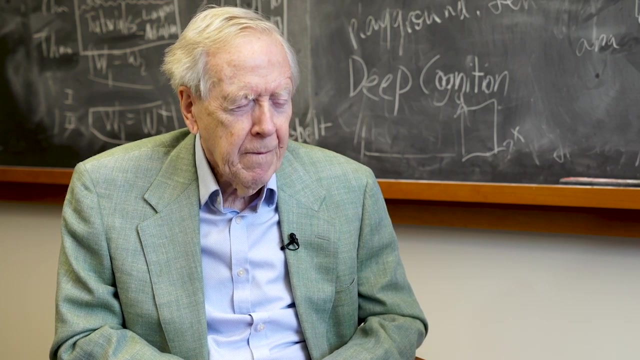 I suppose I try to think it through once again- and and, and that then you sort of automatically see the word, you recognize what words you need to use and what step, what the steps are: Yeah, if you, if you don't, if 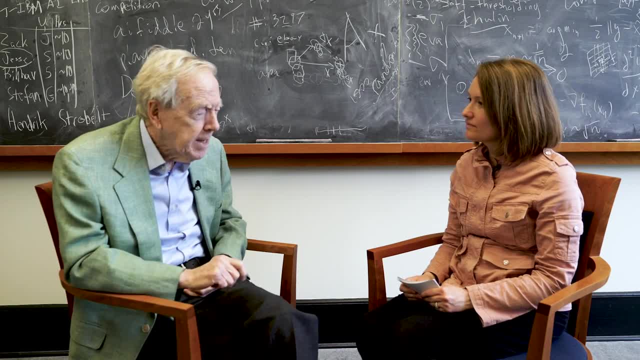 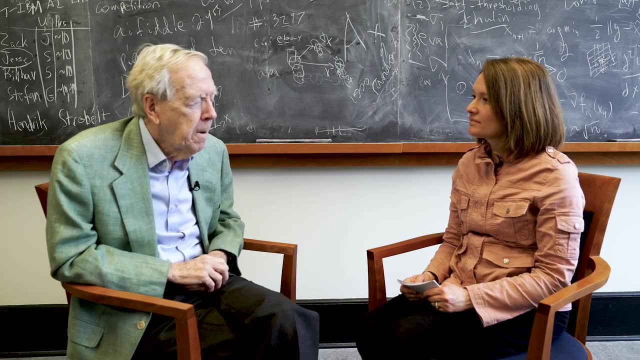 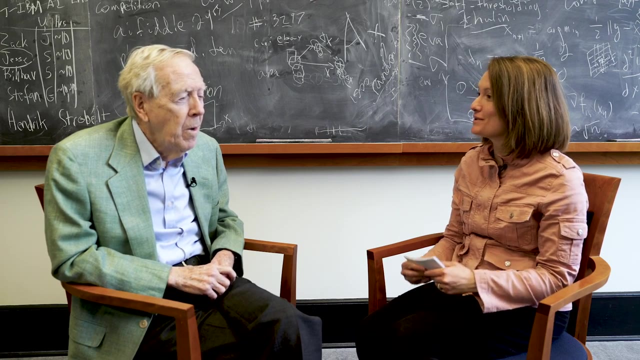 you're not thinking it yourself, then you're probably going too fast and not connecting with the thinking of the class. And how do you connect with the thinking of the class when it's such a large lecture hall? Everyone's at a different point in their understanding.